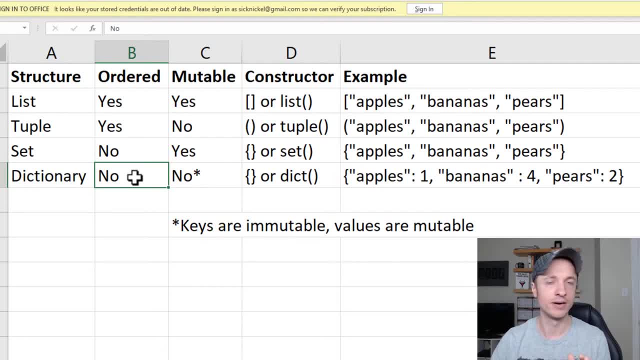 but they're not ordered based off of index positions. Hopefully that makes some sense. Now they are not mutable, kind of as well. So dictionaries are kind of funky because they contain keys and then values related to those keys. So the keys are immutable. 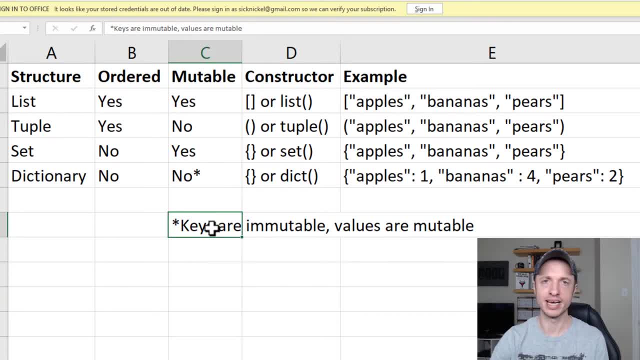 Whatever you set as the key is the key. Okay, you can't go and change the key. However, the values associated with those keys can change and as we go through some examples, you'll see exactly what I mean between keys and values and changing things. 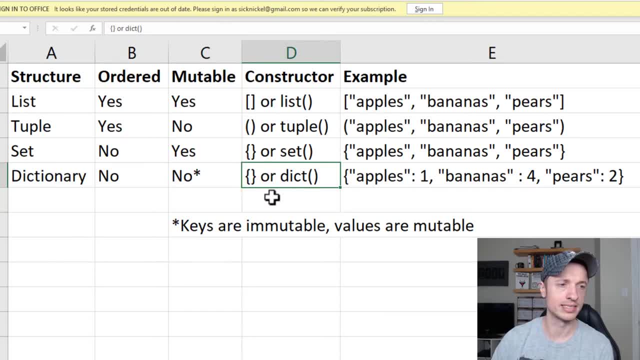 Okay, and then we set it up with the squarely brackets just like we do with a set, but we assign the key as well as the value at the same time, and then Python knows that we're making a dictionary compared to a set. So let's go over and. 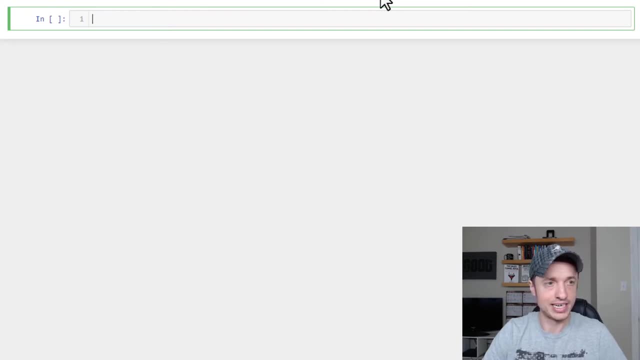 start playing with it. So let's go ahead and create our dictionary real quick. So I'm going to make one called cart cart. like shopping cart, It's equal to squarely brackets, and we'll go with apples. So we'll run it real quick and nothing happened. Let me do print print. 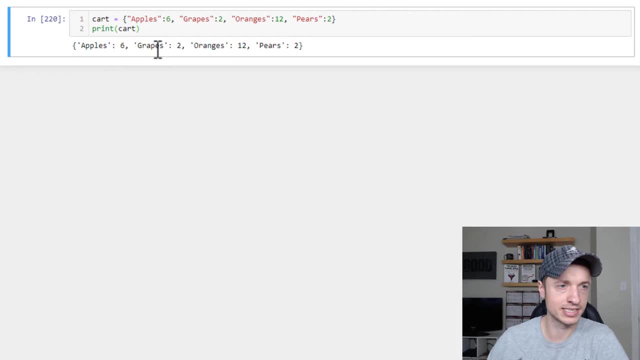 All right, so there is our dictionary: apples of six, grapes of two, oranges of 12,, pears of two. Now if we want to print, like how many grapes we have in our cart or bunches of grapes we have, we can use the print. and then we do cart and we say what we want to print. so 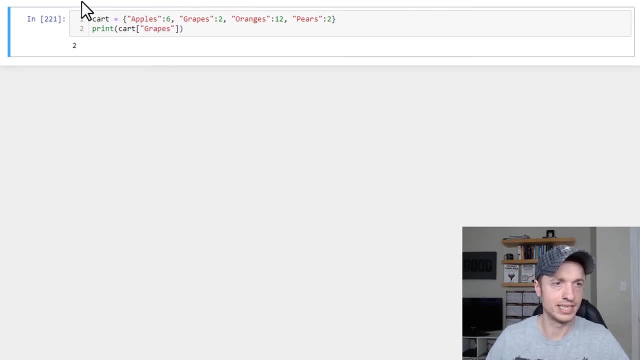 grapes, grapes. So we run that real quick and we see that we have two bunches of grapes in our cart. So basically, instead of using like zero, one, two, three or one, whatever the index is- to call up the, the value we're trying to get, we use the key instead. 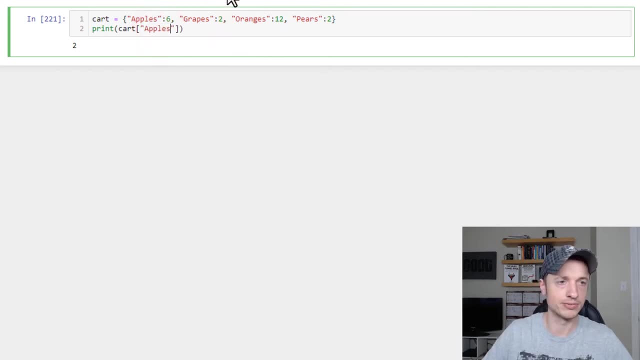 So grapes is the key versus apples. So how many apples we got in our cart? We got six apples in our cart. Now, if we want to add something to our cart, it's very easy to add something to our dictionary, So it would just be our. 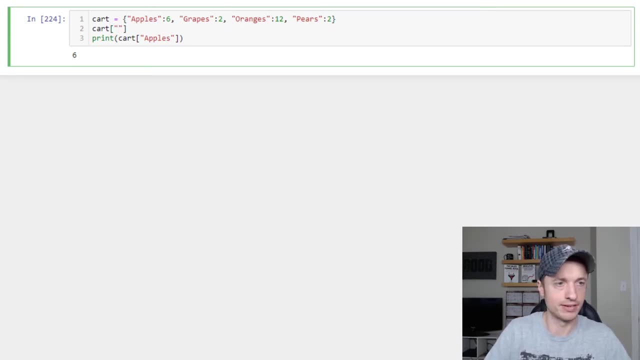 dictionary and then we set our key. So let's say we want to add kiwis, and then we set it equal to whatever we want. So let's say we like kiwis, We want seven kiwis in there, And so now we've added kiwis to our 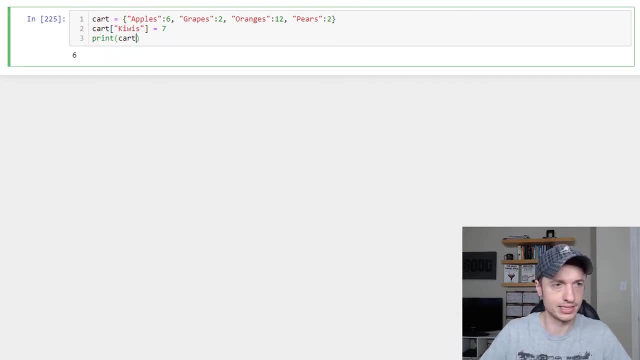 dictionary. Let me go ahead and print out our whole dictionary real quick so we can see. So we got apples, six, grapes two, oranges twelve, pears two, kiwi seven. So that's how you go ahead and add items to a dictionary. Also, we can change the values in our dictionary again. 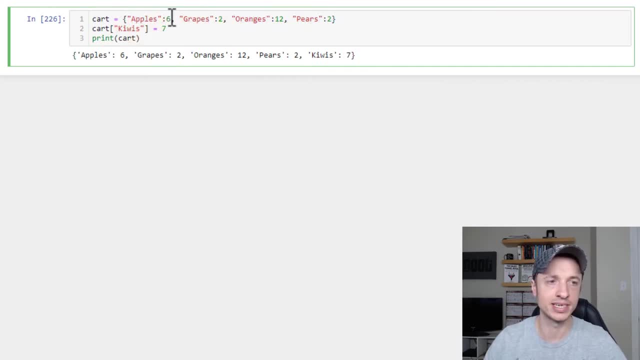 We can't change these keys like apples, grapes, oranges, pears and kiwis, but we can change the value of the particular key. So let's go ahead. Let me delete kiwis out of there and run it real quick, And then let's say that we decided we don't want any apples, so we can set that to zero. 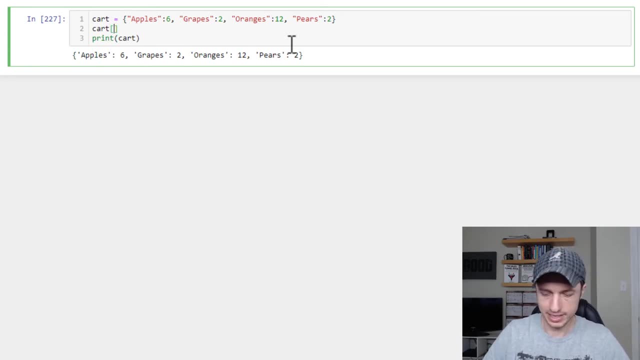 I do a cart and then our brackets here and apples is equal to zero. Run it real quick. and now we've changed the value of our, our key of apples down to zero. All right, Let me go ahead and wipe this out real quick Now. also, the in operator works with dictionary. 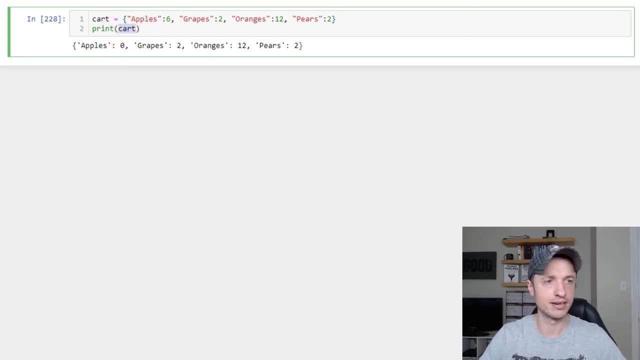 So we can see if a particular key is pressed present in our dictionary. so let's see if apples is in cart. and it came back as false because I can't spell apples correctly and then we got true. so obviously if you spell the word correctly you get a true, assuming it's. 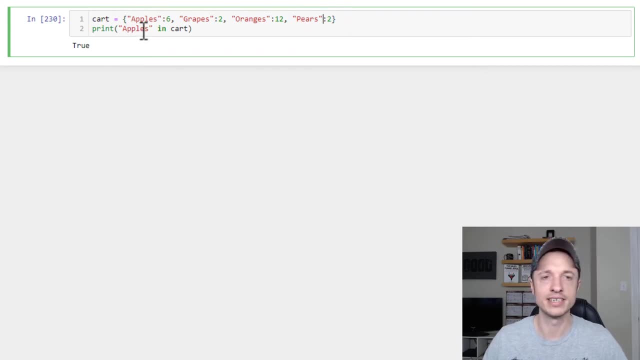 in your dictionary. obviously, if it's not in your dictionary, you get a false. like when I type applies, we got a false statement, so the in operator works there now. one last thing I want to show you is the get method, which is useful for dictionaries, because you can get errors in dictionaries if something, if you call. 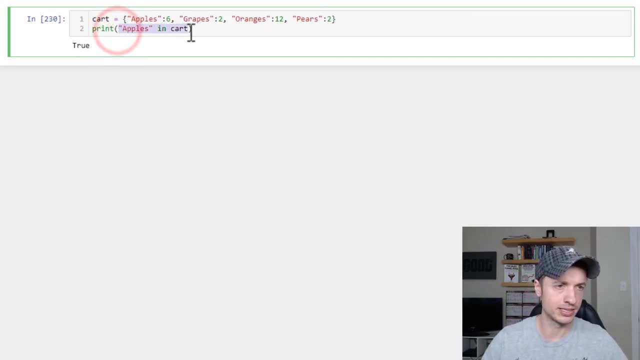 something and it's not there. so let's do this print and we will do cart and apples keeps saying applies. so we got six right. so doing it like this, we get the value of apples. now let me do another example right below it. so if we do, do one,